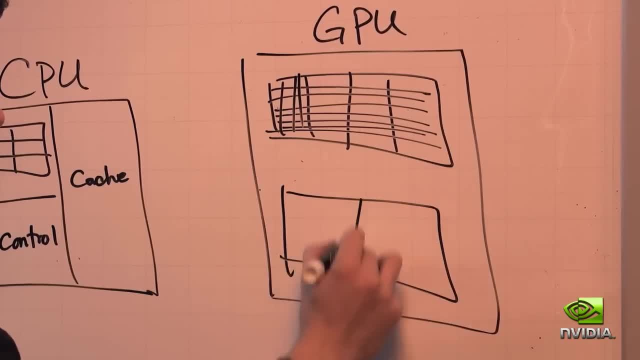 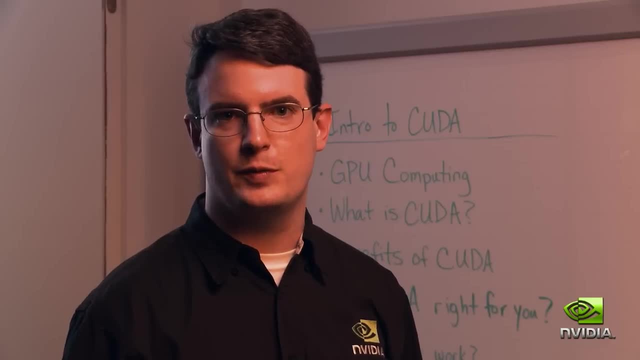 any given moment, simultaneously juggling them. So overall, we have thousands of threads that the GPU is working with at any given time. So CUDA provides a scalable, intuitive way to express parallelism. We simply write a program for one data element and it gets. 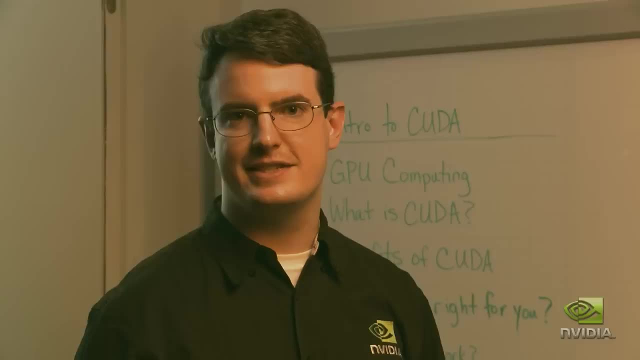 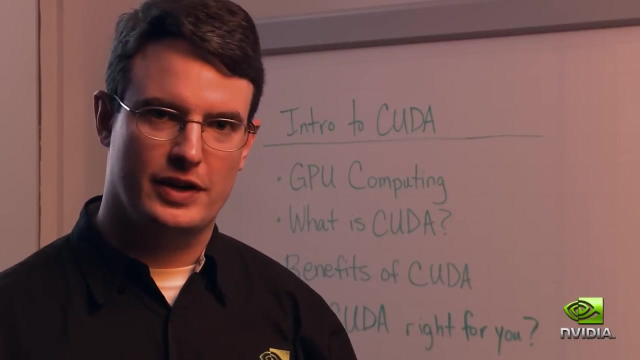 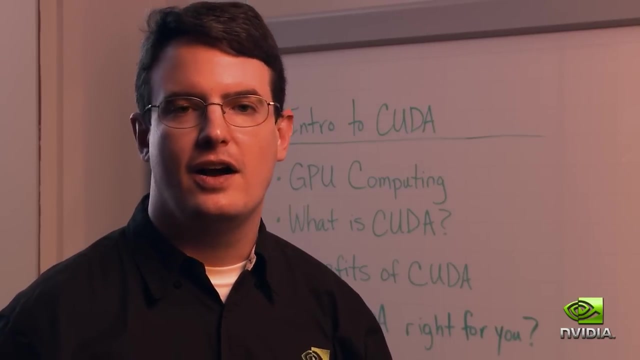 automatically distributed across our hundreds of cores for thousands of threads. So is CUDA right for you? Well, what kinds of workloads does your application require? If you have a task oriented application, for example one that needs to update five records in a database, then GPU computing probably isn't the right choice. On the other, 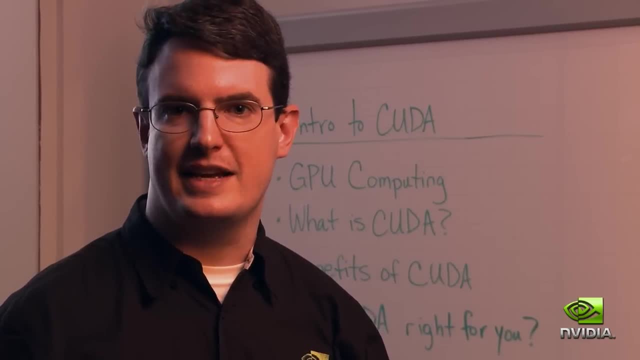 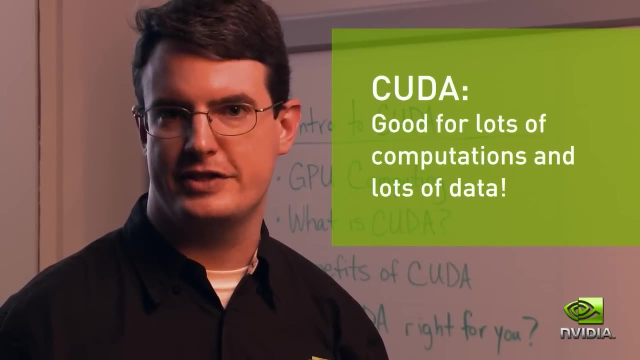 hand. if you have a large amount of data that you need to process- for example, searching through a terabyte of data for a string or a massively parallel molecular simulation or engineering simulation- then GPU computing can be a very good fit. The hundreds of cores. 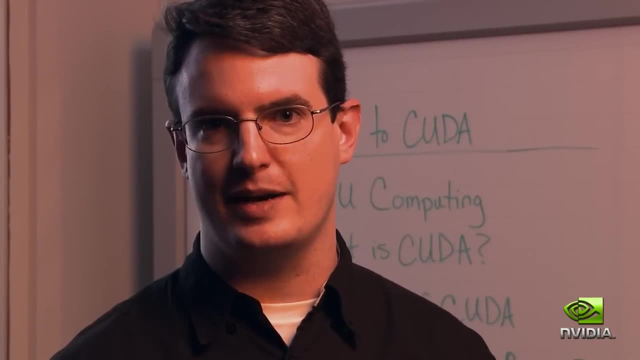 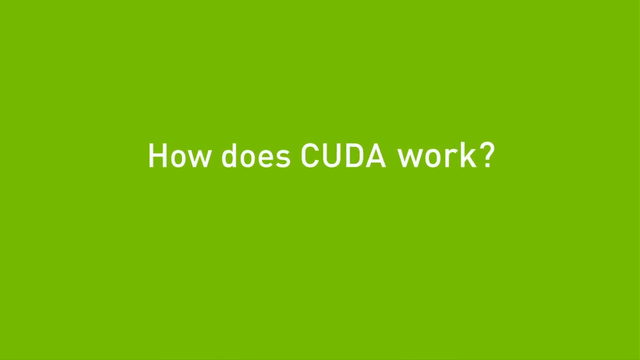 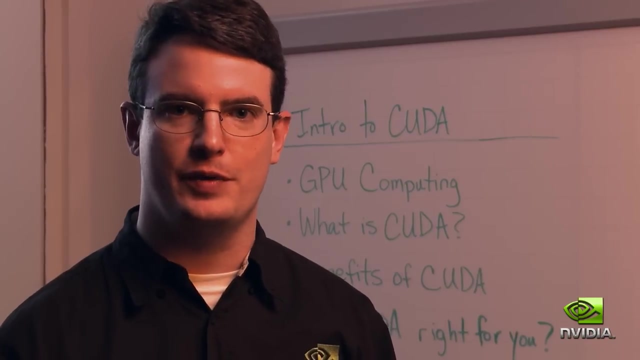 of the GPU give us a high throughput way to process our computing job, And most of the interesting compute tasks these days are throughput problems. So how does it work? Well, the days of free scaling are over. you have to go parallel. so CUDA gives you a way that you can express parallelism in a way that will scale with. 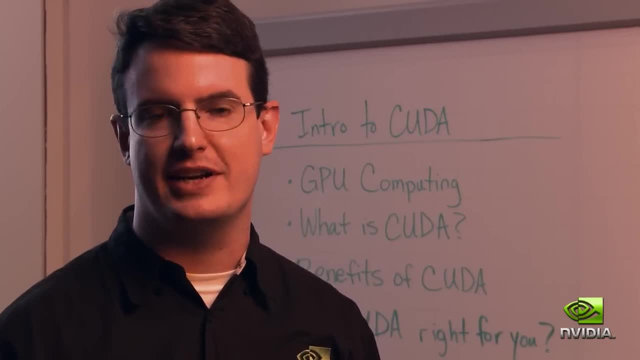 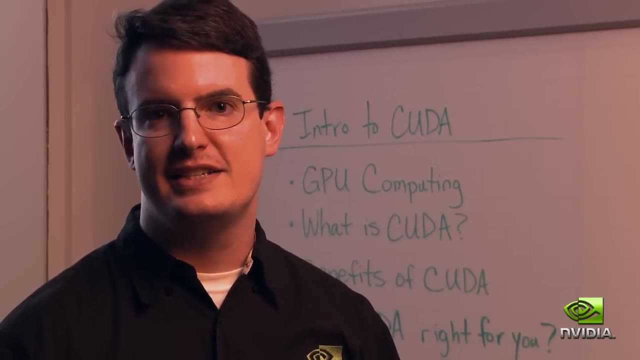 future architectures in languages you already know, like C, C++, Fortran and so on. It will allow you to take advantage of libraries like our BLAS and FFT libraries and others to get best in class GPU performance, And it will give you an ecosystem of developer tools and 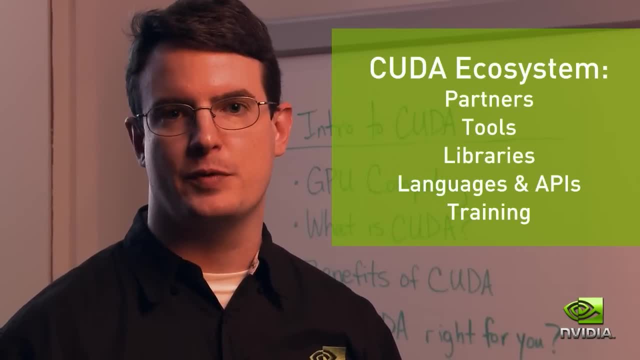 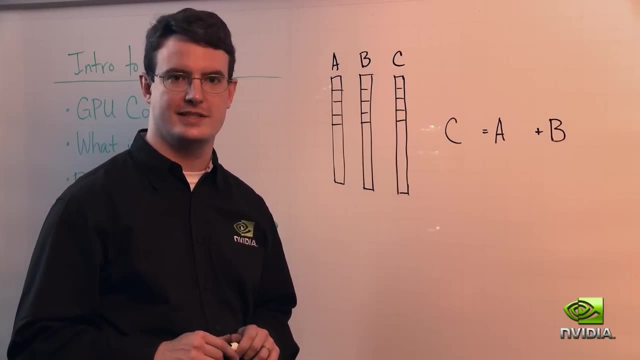 solutions that allow you to fine tune your own code to get best performance out of the GPU. So let's take a look at an example that will show how it is that CUDA makes it easy for us to express all this parallelism we've been talking about. Consider a case where 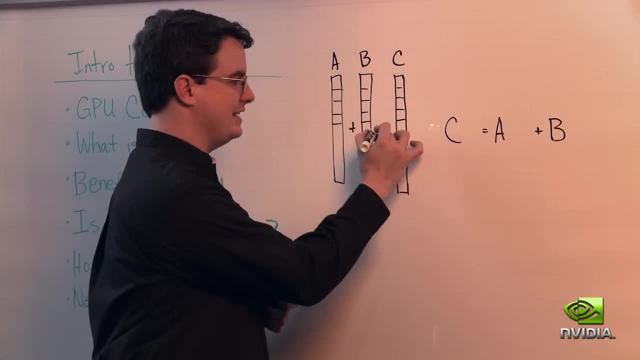 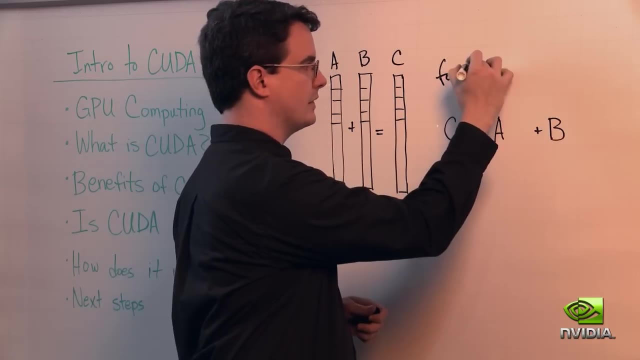 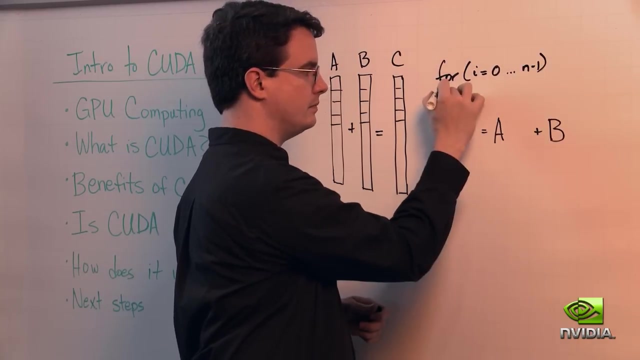 we have three vectors, A, B and C, And we simply want to add these vectors, A and B, and store the result into C. Well, in C. normally in the sequential case, this would simply look like a loop that says: for i equals 0 onto n minus 1, where n is the length of the 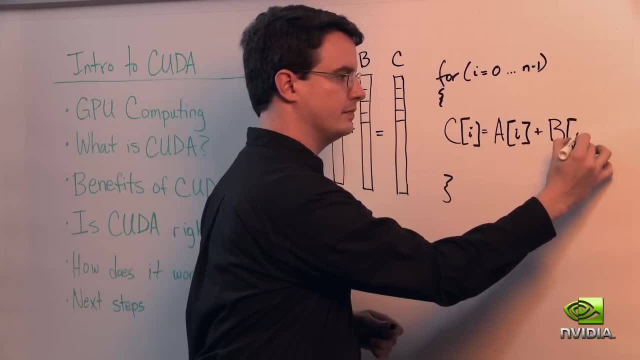 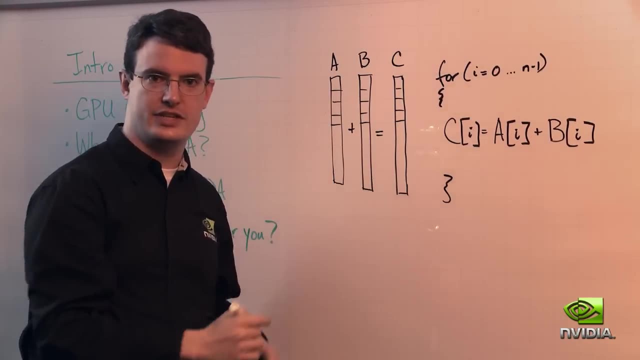 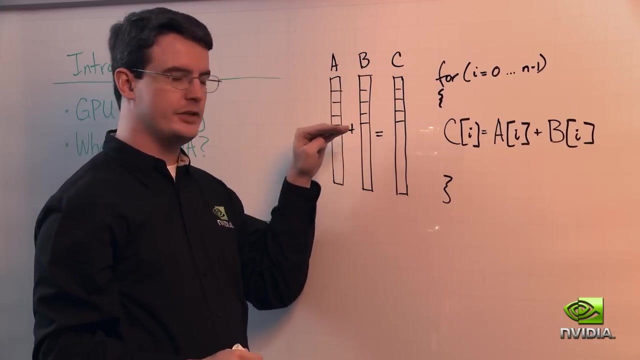 element, Then one element at a time. I add the zeroth element to the zeroth element, and then the first, and then the second, and so on down the chain, one at a time, in series. So in CUDA instead, what we consider is each of these individual additions is a thread.